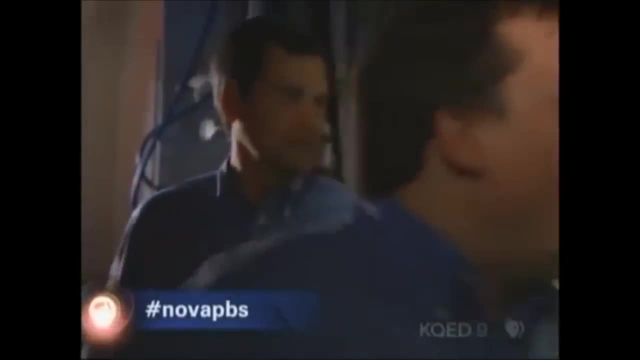 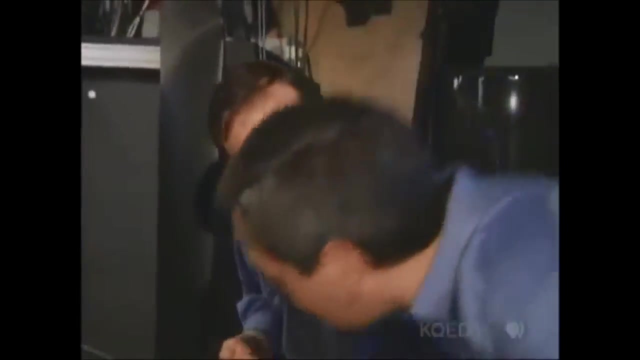 A place so clear and cold physicists can see the fundamental laws of nature in action. MIT's Martin Svirlein is going to use sodium atoms to show me how to get there, the final frontier of cold. Wow, And so how do you do that? 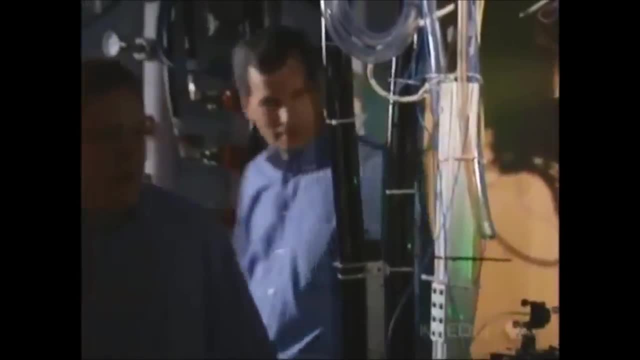 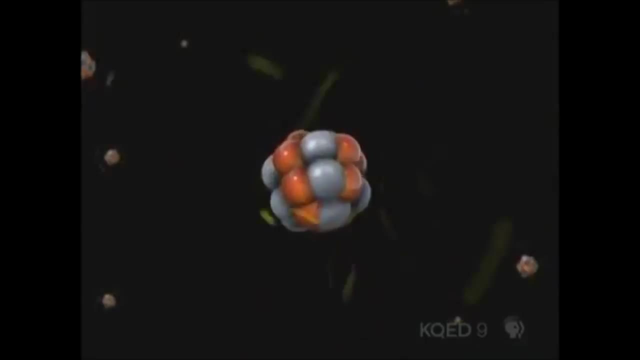 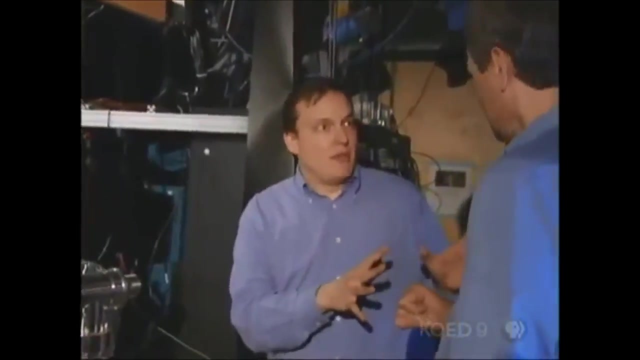 So we can start over there at the oven, The oven Step one. cook up some sodium atoms the same kind in your table salt to about 700 degrees Fahrenheit. That way you can separate them. You want to get single atoms to play with single sodium atoms. lots of them, a whole stream of them. 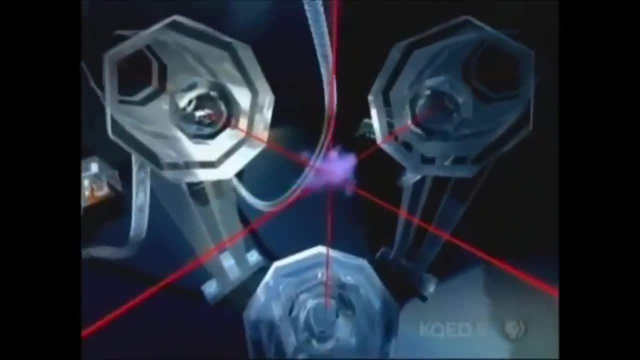 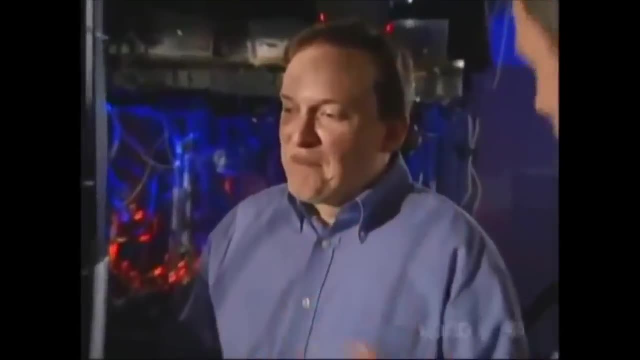 Step two: hit them with lasers. I know you MIT guys have the reputation of being very smart, but I have a little tip for you. Lasers are hot. You might be a little backwards there. Yeah, you might think about Star Trek, where they kill people with lasers. 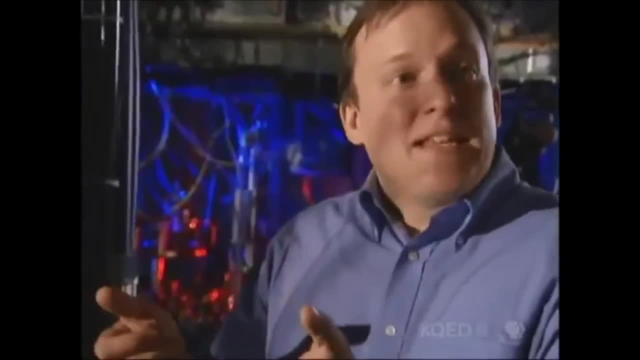 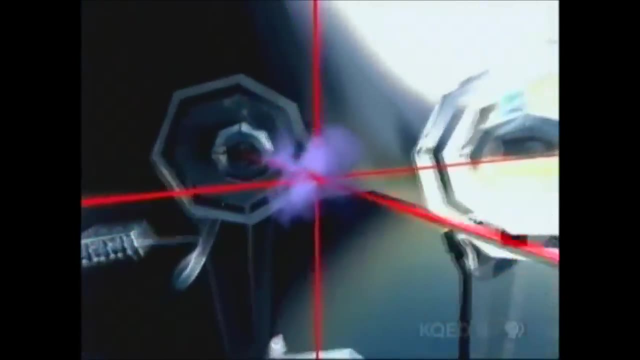 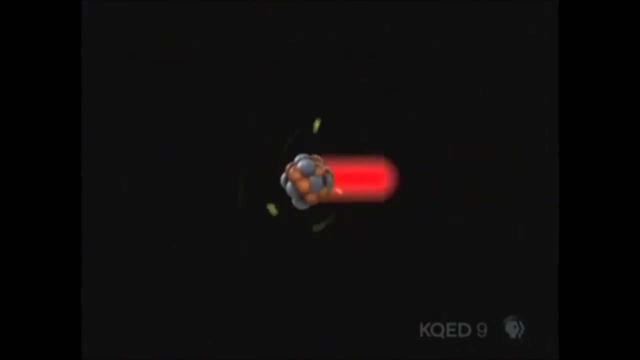 Turns out here. we cool atoms down with lasers and they get a recall from it. Just if you hit a billiard ball with another, That's a billiard ball. In other words, when you hit atoms with just the right amount of laser light, it acts like a little shove in the opposite direction that the atom is moving, slowing it down. 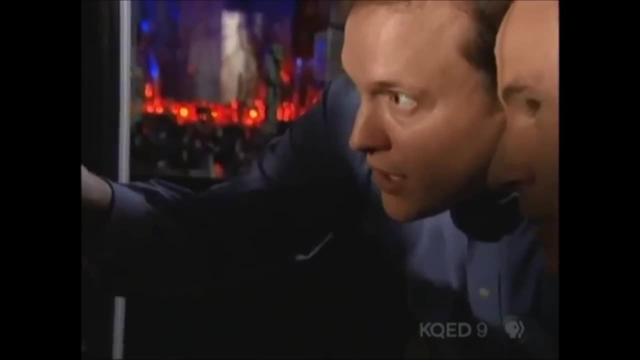 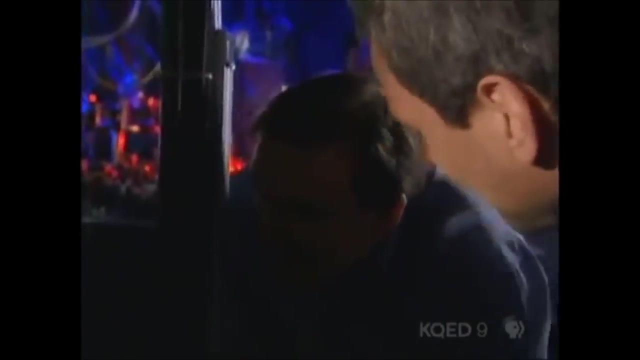 If you look down here, you will actually see the cold cloud right there in the center of the vacuum chamber. So that glowing star thing, It looks like the sun. It ought to be super, super hot. No, it's actually extremely cold. 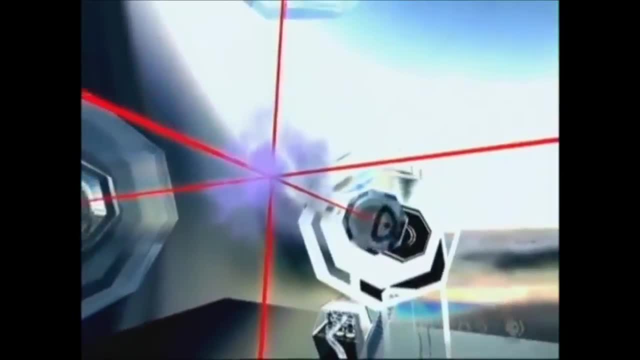 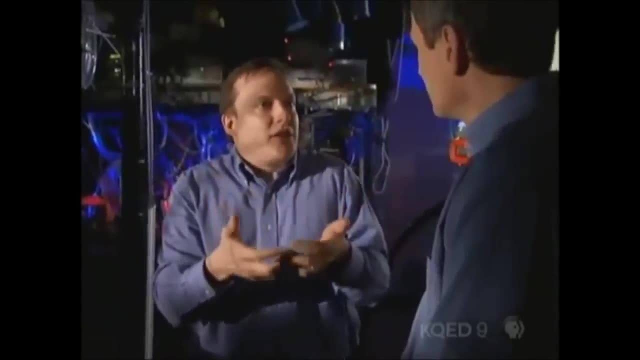 Those are a billion atoms cooled to a milliKelvin, A thousandth of a degree above absolute zero. But lasers can get us only so far. You cannot reach the nanoKelvin temperatures just with laser cooling, So we need another technique. 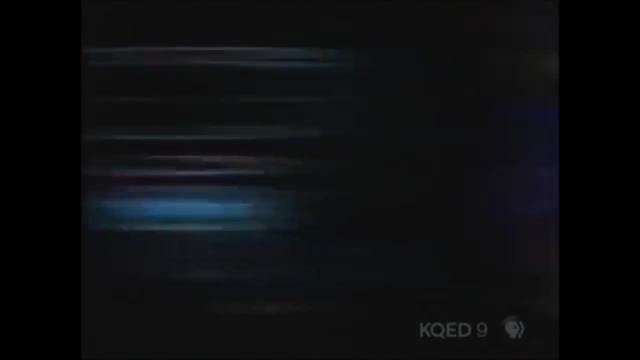 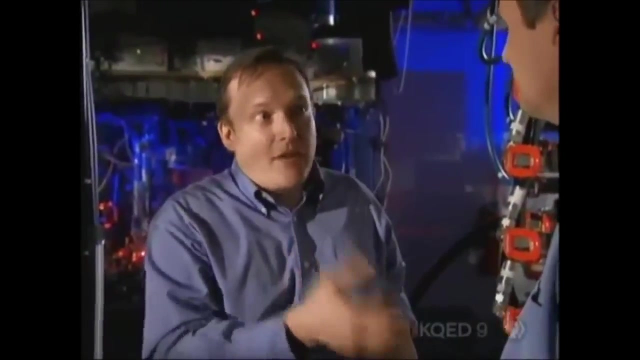 Which brings us to step three. Get out your coffee cup. What takes over after laser cooling is what we call evaporative cooling. It's the same thing that happens to your coffee right now, because it's just cooling down. So if you now force it a little bit by blowing on the coffee, 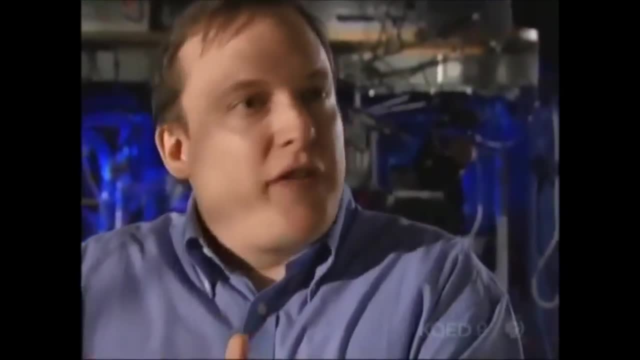 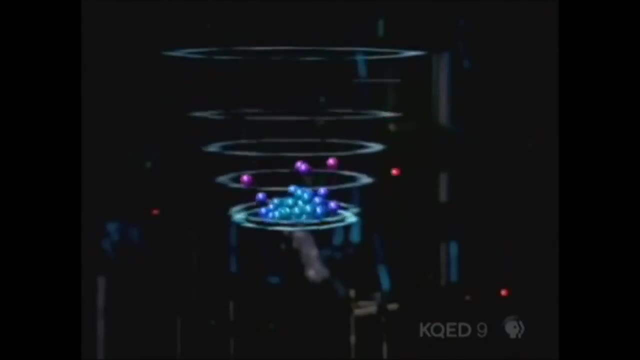 you speed that process up, the coffee gets cooled more quickly. That's exactly what we do here, But instead of a coffee cup, Zierlein uses a cup made of magnetic fields to trap his atoms. Then he blows on it with radiation and lowers the rim of the cup to let the hotter atoms escape. 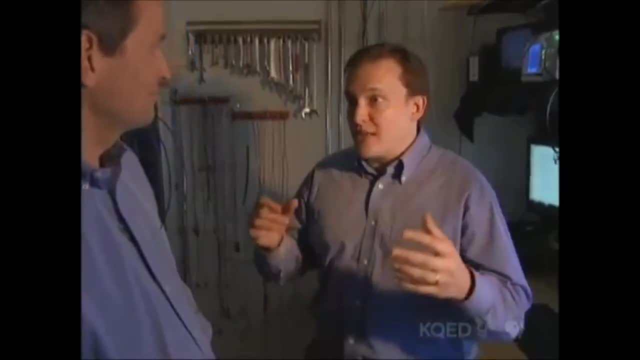 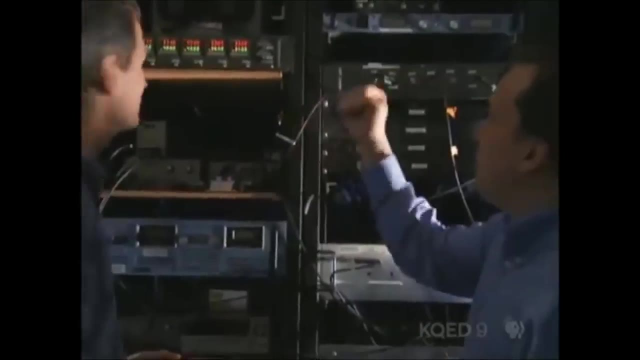 So now we're going to do this coffee cup cooling, It's going to bring us to nanoKelvin. Okay, Ready for this? Yes, Let's do this. Can you please switch on this stuff? Do this, This is great. 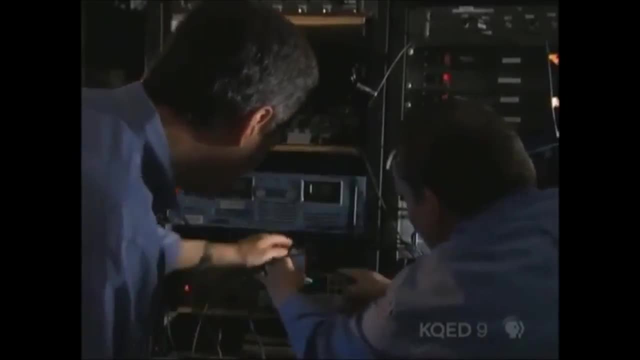 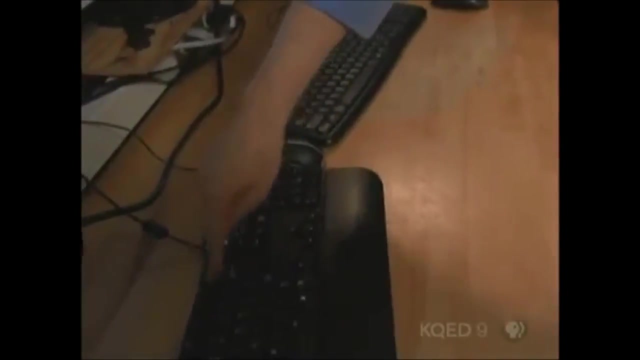 Let's switch on this guy. And then this awesome knob here, Press the awesome white button. Fantastic, So that's good. Please press F12.. Always wondered what F12 does. So you see now the atoms are cooling because the cloud size gets smaller and smaller and smaller. 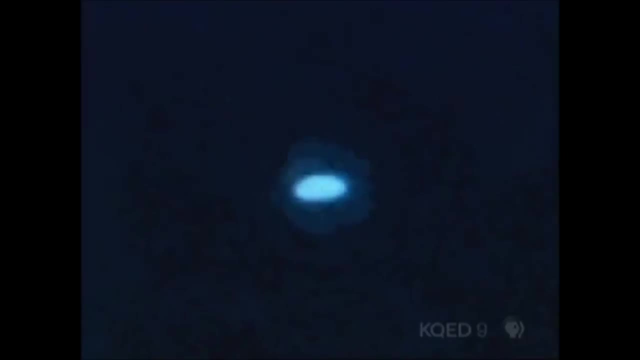 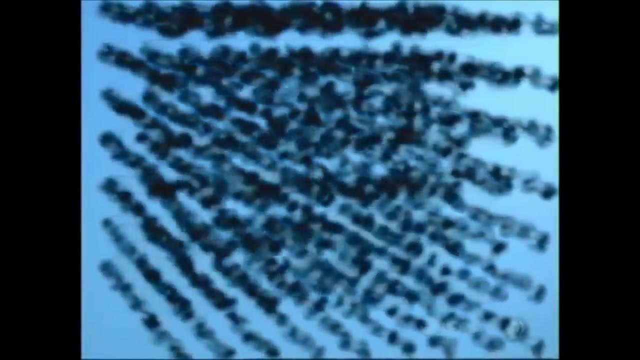 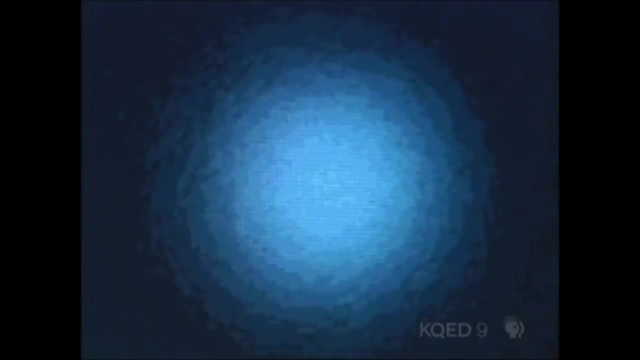 Here you see the temperature drop, drop, drop, drop, drop. Oh wow, It takes a few minutes, But eventually the atoms become so cold they lose their individual identities altogether and coalesce into that new state of matter called a Bose-Einstein condensate. 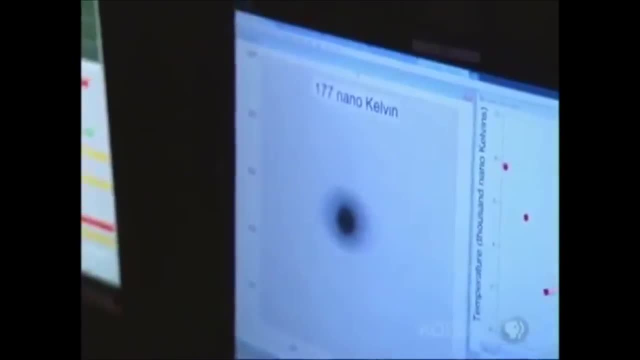 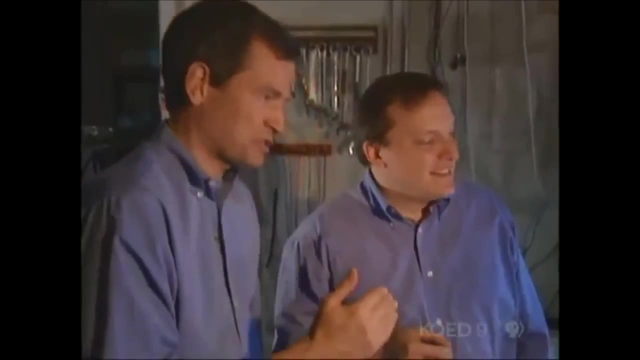 Wait a minute. wait a minute. Okay, So that's the condensate. That's the condensate, But look at the temperature. Yeah, It's very cold: 177 billionths, Billionths of a degree, 177 billionths of a degree Kelvin. 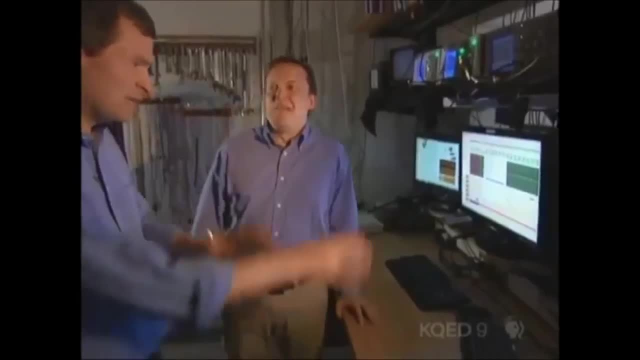 This is the coldest spot in the universe right now. That's amazing. So not even in outer space. No, no, no. Outer space is a million times hotter. Not the dark side of the moon, No, it's like all hot. 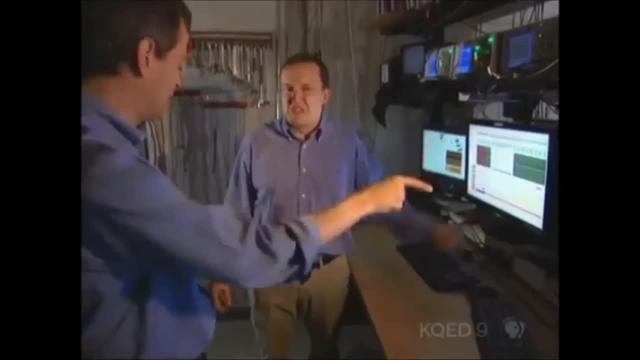 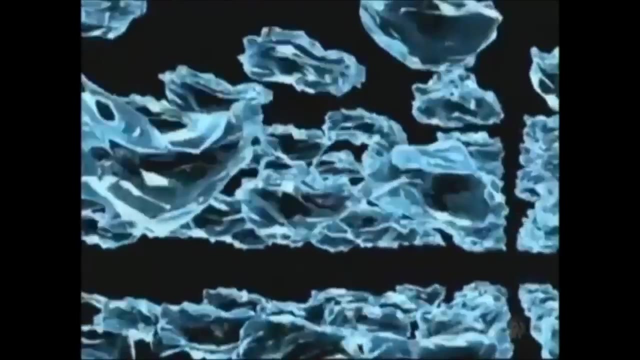 Comets Terrible. Yeah, Black holes, Nothing. This is it. This is it In this room? Yes, That's amazing. I would ask it's autographs if I could. But it's not about setting obscure records. 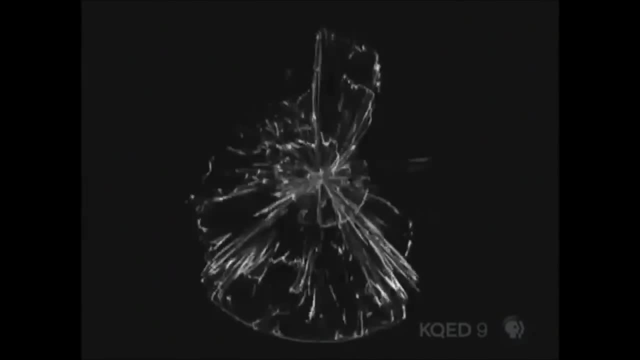 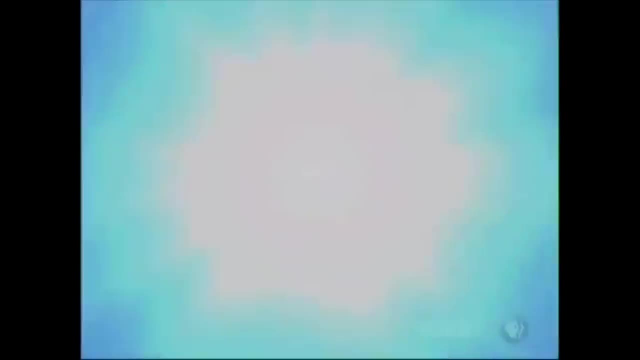 What SphereLine is excited about is what these exotic states of matter can teach us about the universe. Our puff of gas teaches us about the neutron stars, or a split second after the Big Bang, There was this weird form of matter called the core gluon plasma. 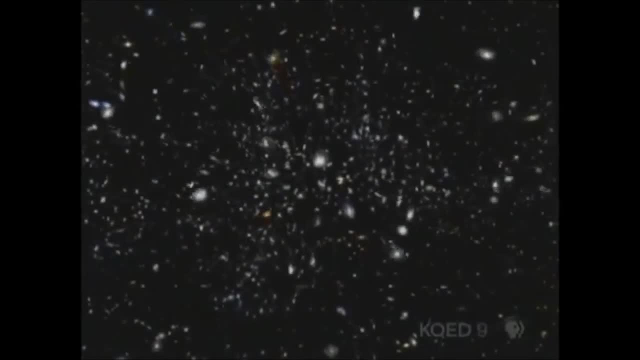 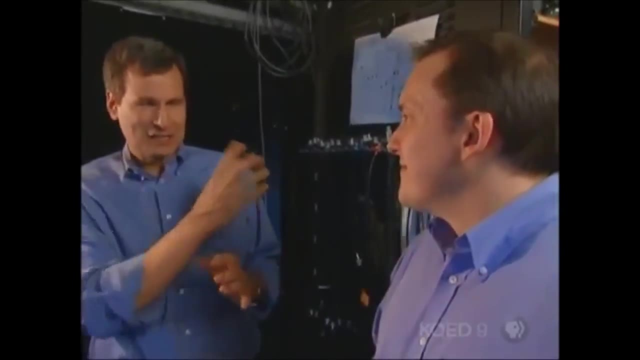 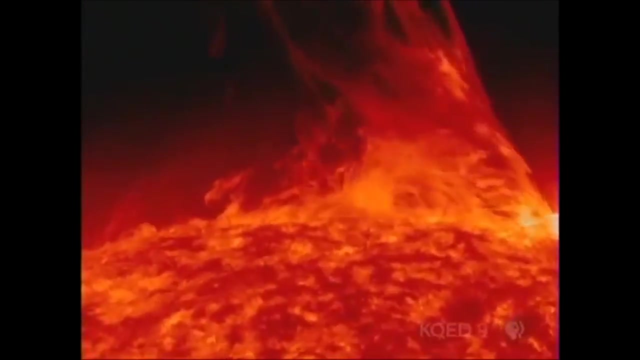 A super hot type of matter in the early universe that would give rise to everything we see today. So you're telling me that this tiny freezing cold dot can teach us something about enormous blazing hot stuff. That's the fun part of physics: It connects these very different areas. 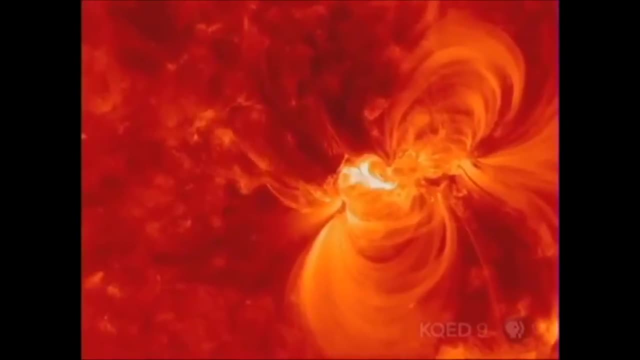 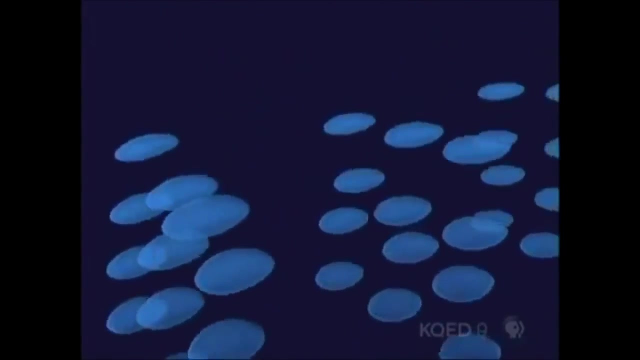 They're very hot, very cold. Everything is governed by the same laws. Amazingly, what happens at this point in time, Amazingly, what happens at these ultra cold temperatures, is that atoms get so smeared out their waves start looking indistinguishable from those of super hot particles under extreme pressure.